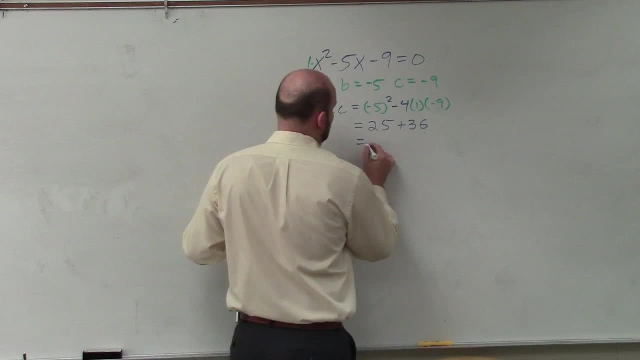 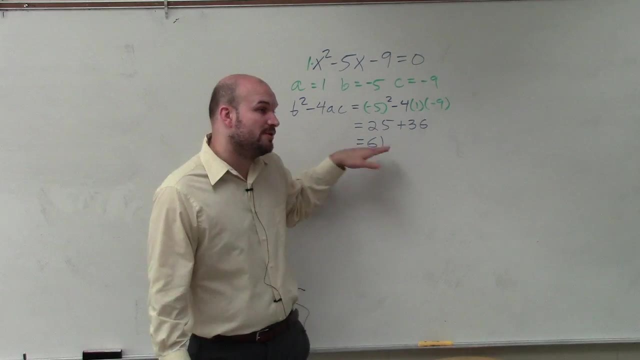 Yes, So therefore that equals 61.. However, the question is not to find the discriminant. The question is saying what is the solutions? However, by knowing what the discriminant is, I determine that that is not a square number. 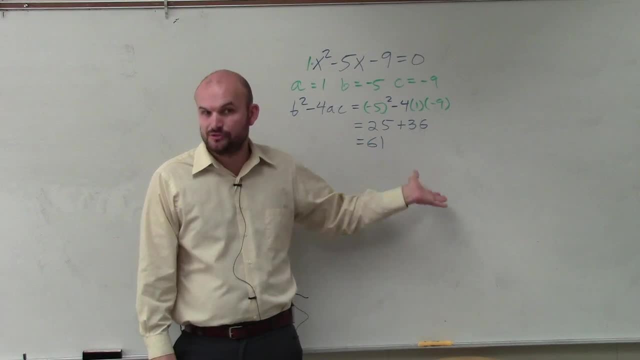 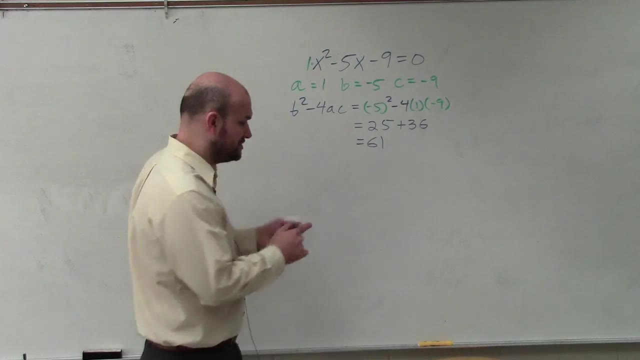 So therefore, I am going to have two real, irrational solutions. You should just know that in your head by studying from those notes. If they ask you, that's what you would answer, But they're asking for the solutions. So to find the solutions, remember x equals is going to be our solutions. 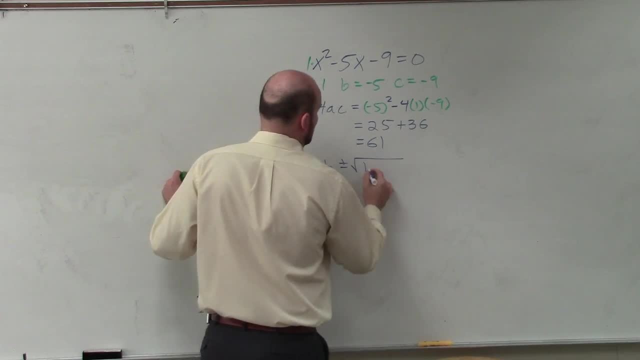 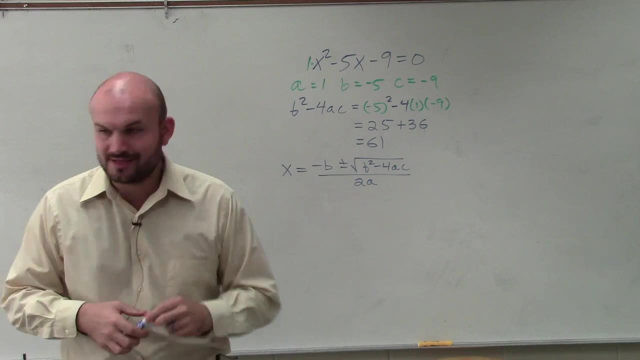 Opposite of b, plus or minus square root of b, squared minus 4 times a times c, all over 2 times a. That's the quadratic formula. We need to know it. We're not going to do it. We're not going to sing a song to remember it. 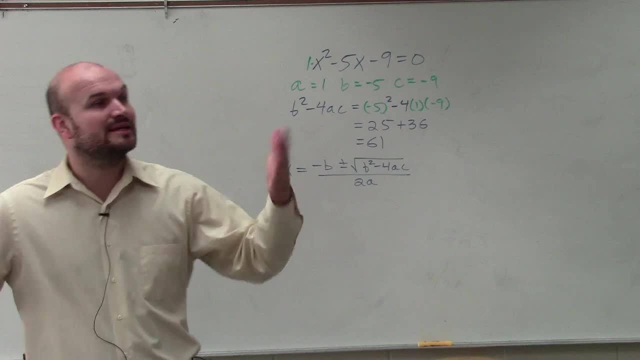 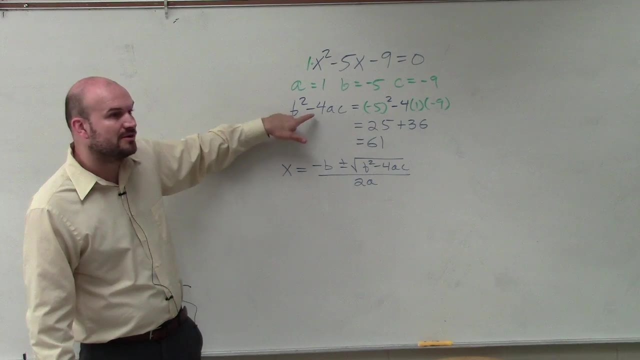 You just need to make sure you memorize it, Write it down in the mirror in your bathroom and keep on saying it over and over and you guys will be good. The nice thing about this- at least the quadratic formula- is, if you guys remember, b squared minus 4 times a times c. 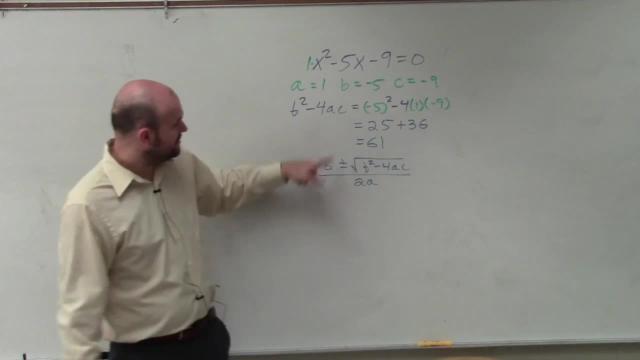 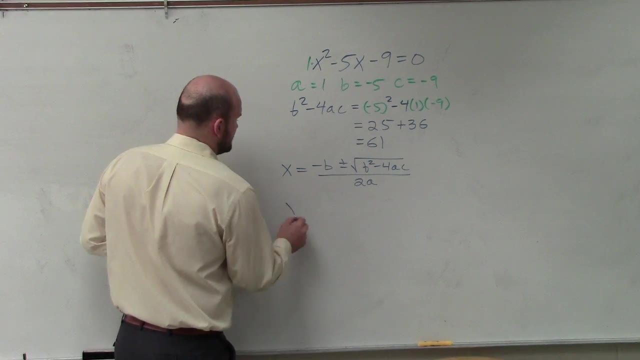 you understand that. that's what goes under the radical. All you need to do, then, is do the opposite of b. So since b is negative 5, our opposite of b is going to be positive 5.. So x equals. basically, it looks like this: 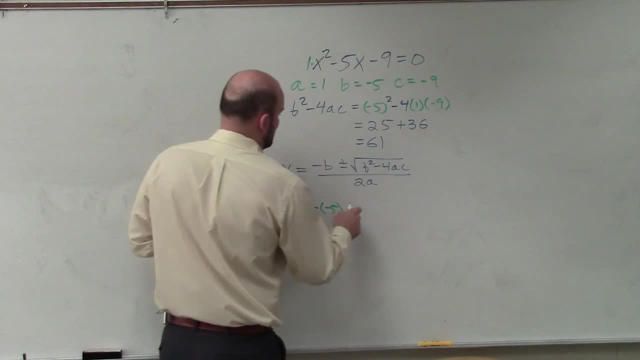 It's opposite of negative 5.. Negative 5 plus or minus the square root. Well, we already know: b squared minus 4 times a times c is 61.. Let me make this green so you guys can see the color code Divided by 2 times a, which is 1.. 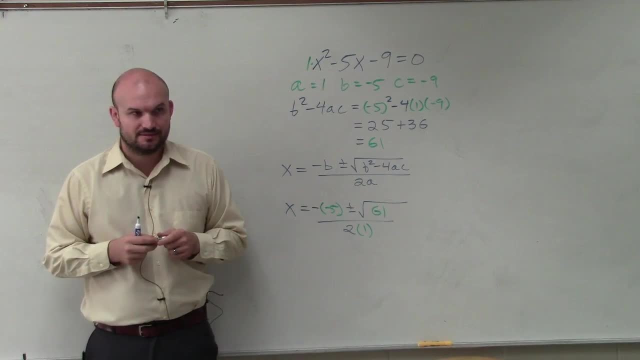 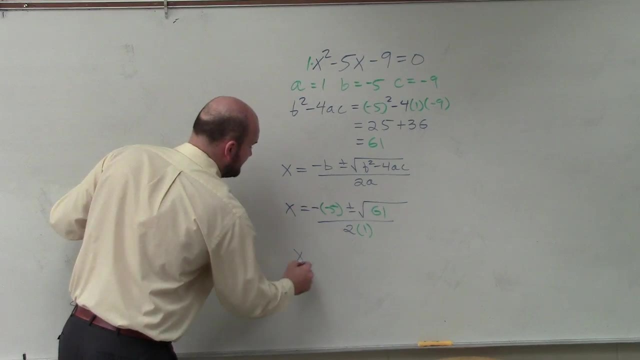 Does everybody see how I plugged in all that information? Yes, No Questions. Good, So now we just simplify. Well, opposite of negative, 5 is going to be 5, plus or minus. I cannot take the square root of 61.. 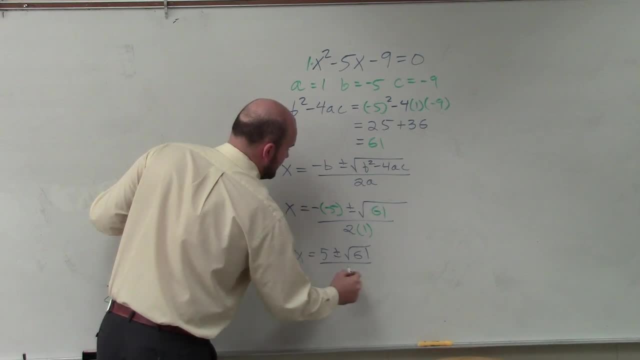 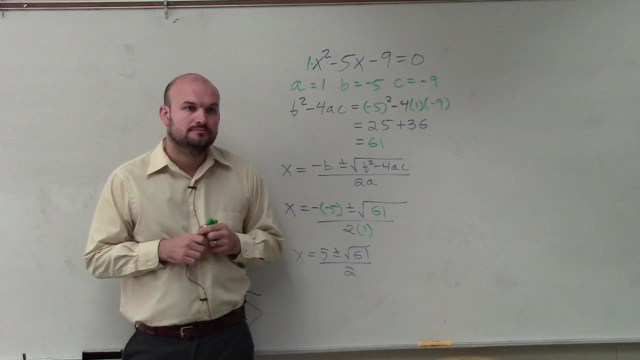 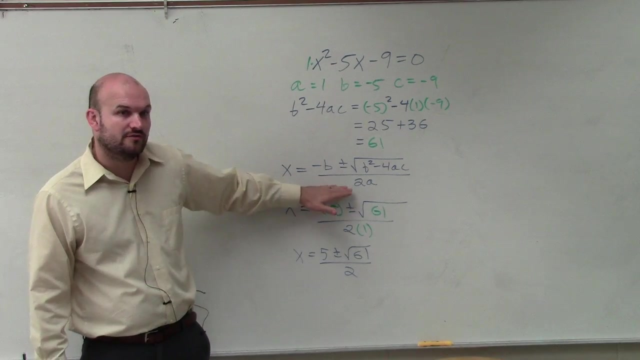 So I'm going to leave it like that And then that's over 2.. Okay, Yes, When you're finding the solutions of a quadratic, you are using the quadratic formula. This problem was the first seven problems that I asked for. 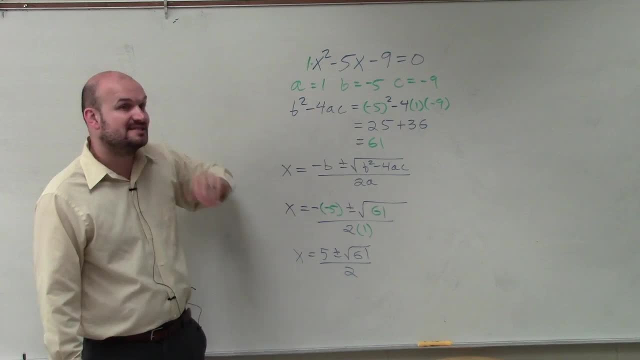 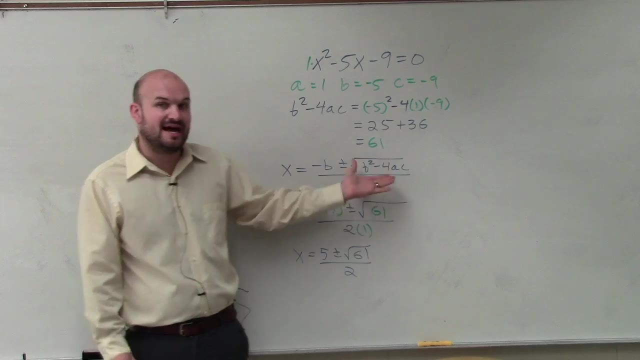 This is what I asked you to do, where it says: just find the discriminants. For the last six, it says: find the solutions. What does x equal? So you have to plug it into the quadratic formula. So for the last six problems. 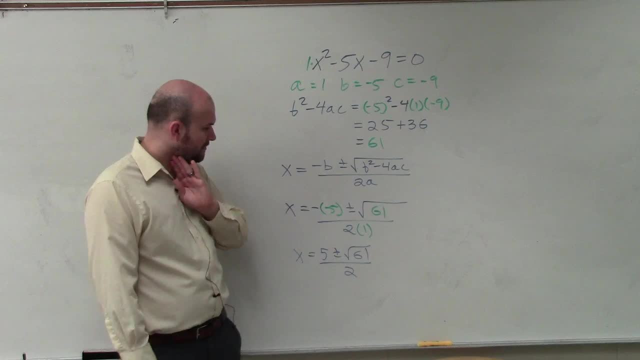 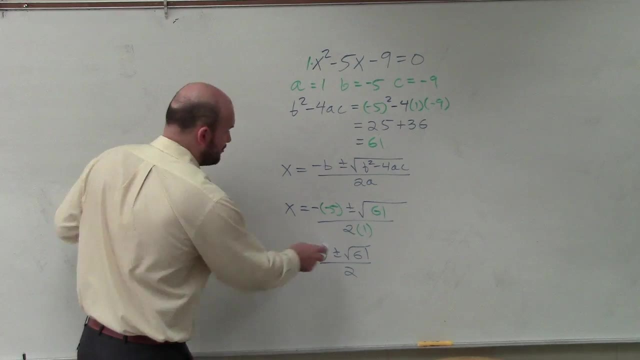 you're using this formula for all of them. So now that is a correctable. that is a correct way to write the problem. You could also break up the plus or minus and you could say x equals. you could also write it. 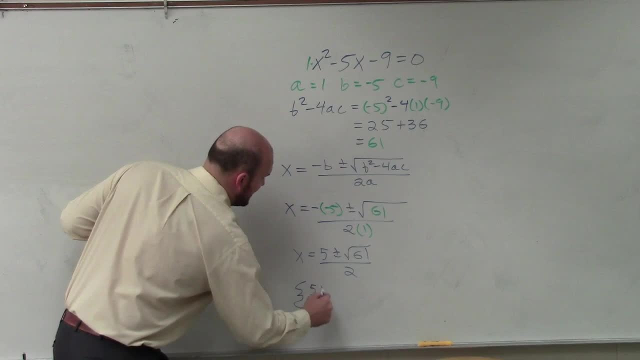 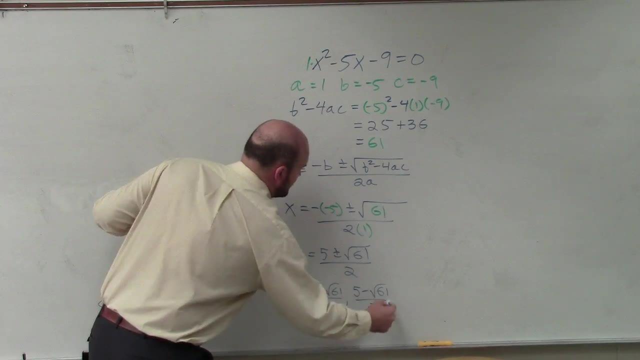 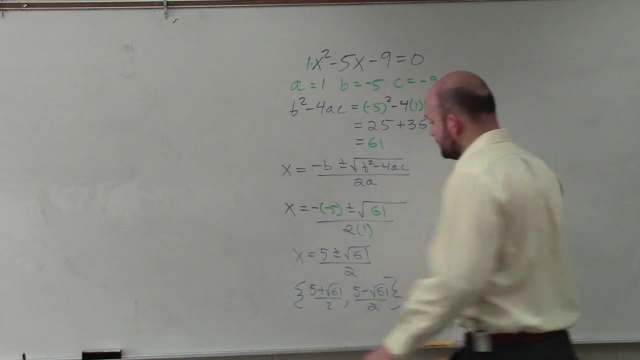 as a plus or minus In a solution set like this: 5 plus the square root of 61 over 2, comma: 5 minus the square root of 61 over 2.. Those are both acceptable solutions. One last thing also to understand. 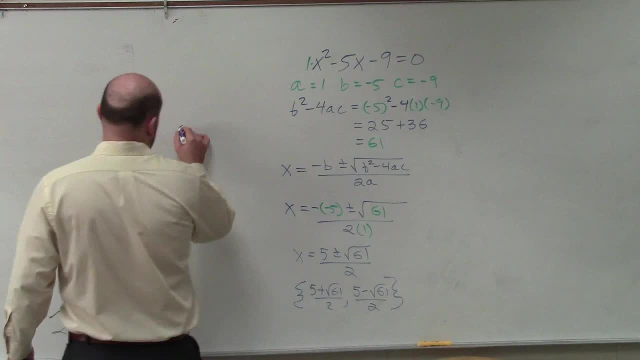 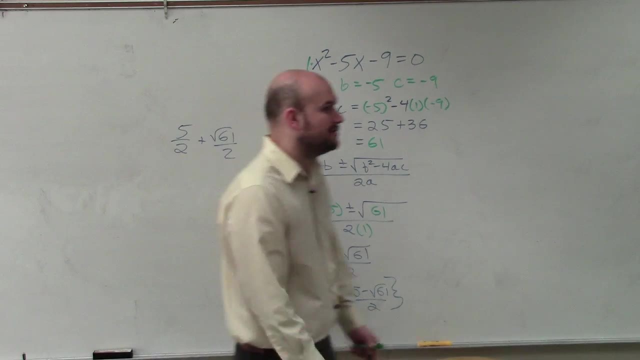 you can also divide the 2 into both of those terms. So it could also look like this, And I'm just telling you guys this because, you know, I don't really know how the answer is going to look. But these are all. 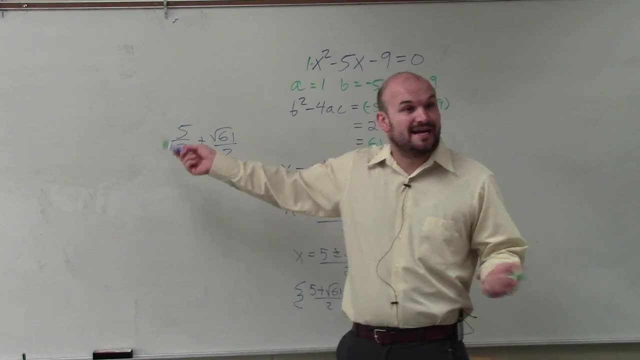 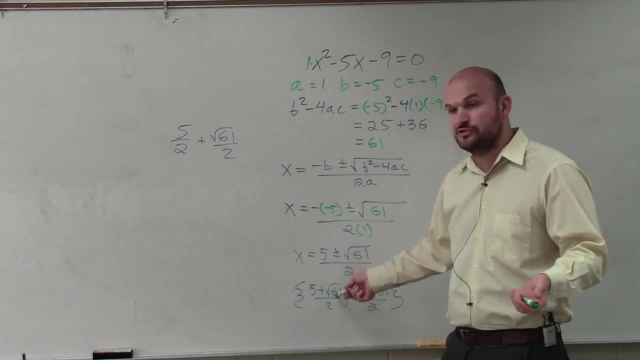 These are all acceptable ways. You can also divide the 2 into both of those And if it can be simplified- usually that's what we do In this case- they can't be simplified. You can't divide the 2 into the 5 or the 2 into square root of 61.. 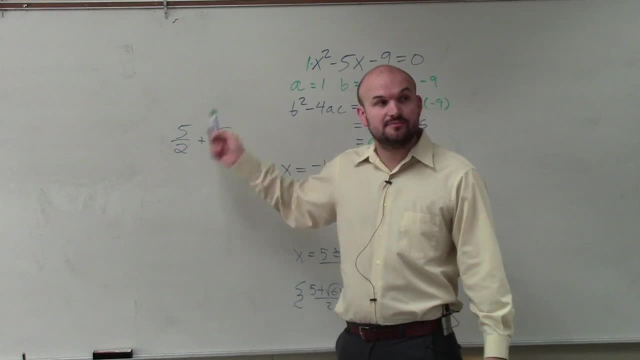 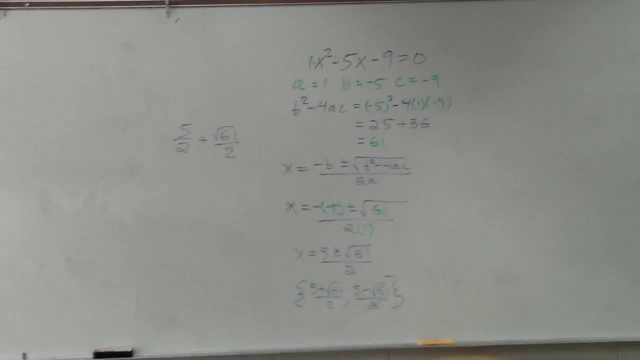 So leaving it like that is perfectly fine. However, if it is something you can divide into, that's another way to write those numbers or the solutions. Okay, All right, Did. 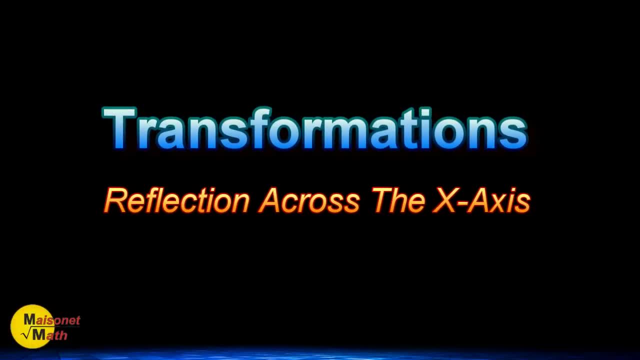 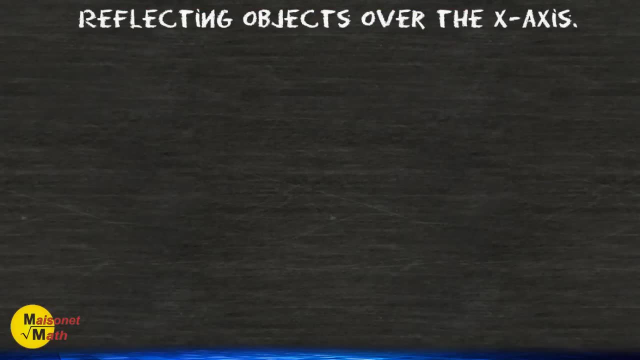 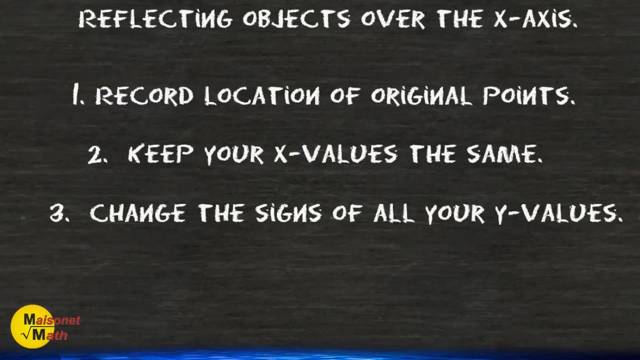 In this tutorial we are going to practice reflecting an object over the x-axis. The first thing that we are going to do is record the location of our original points. The second thing we are going to do is make sure we keep our original x values for each ordered pair and the only.